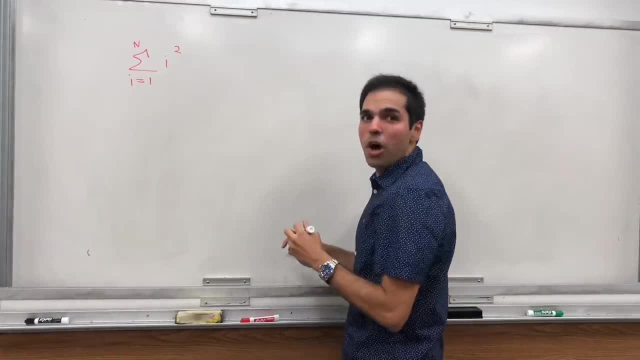 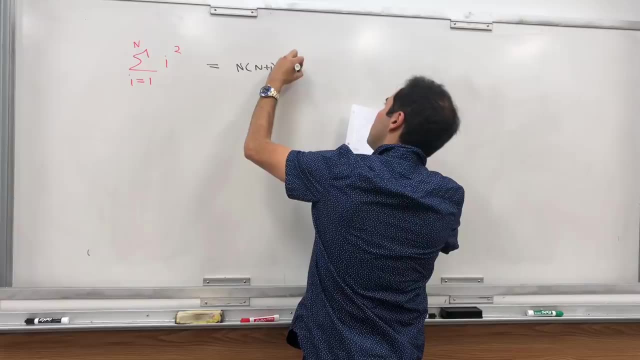 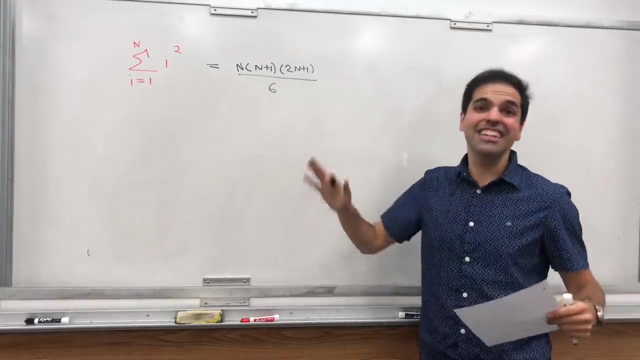 about was a really cool way of calculating the sum of squares. so if you know this formula, it's n times n plus 1 times 2n plus 1 over 6, and usually they do it with induction, but it turns out there's a very easy way of actually getting this formula, so let me tell you about it and you. 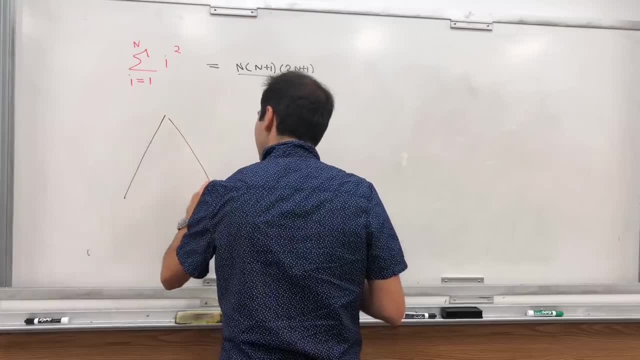 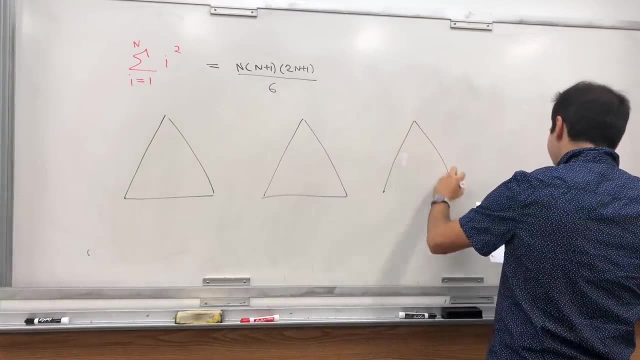 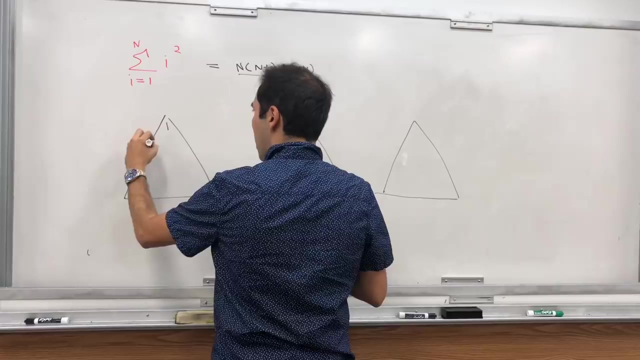 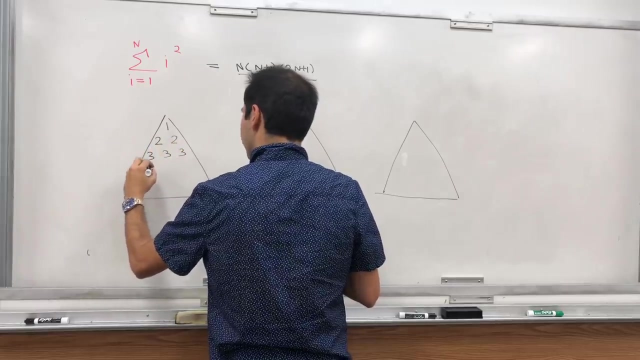 might not believe me, but it is true. consider three triangles. I am such a tease, okay, but don't worry, just wait for it on the wall. first triangle: you start with one and then just go down like this: one, two, three, up to n, and all the rows are the same. so one one. 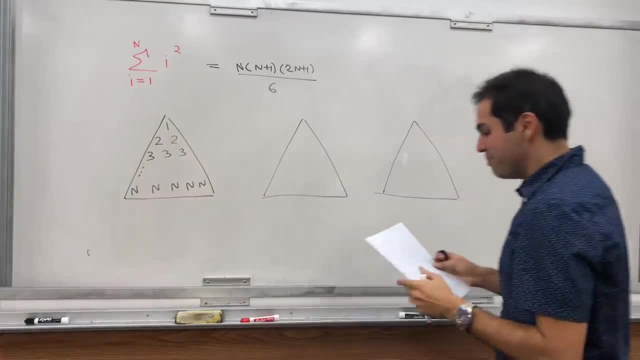 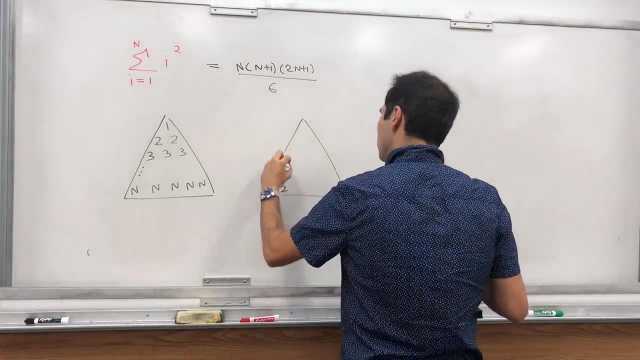 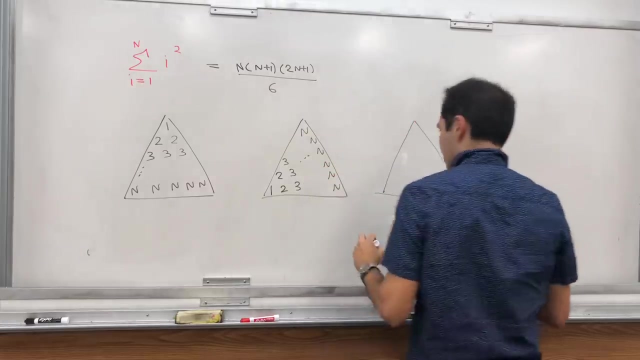 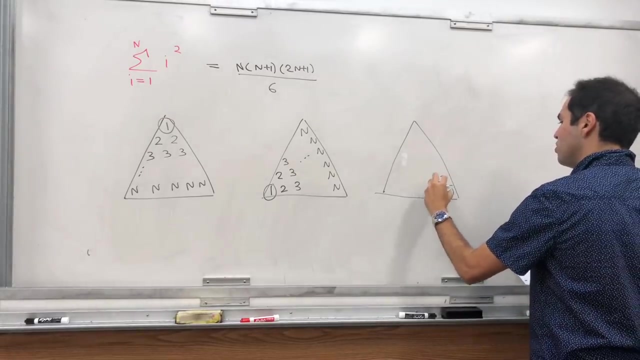 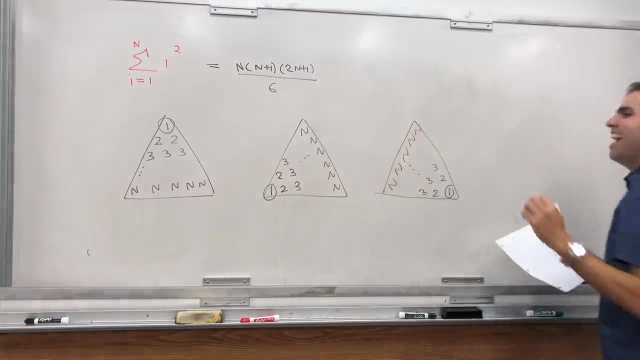 one, two, two, three, three, three, and then, and then right on the other hand, you do the same thing, but you start here. so one, two, two, three, three, three. so if you start here, then you start here and, lastly, you start at the other corner. one, two, two, three, three, three, anyway. so okay, now what is the 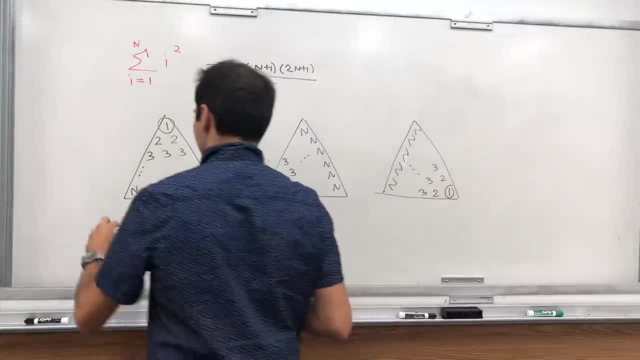 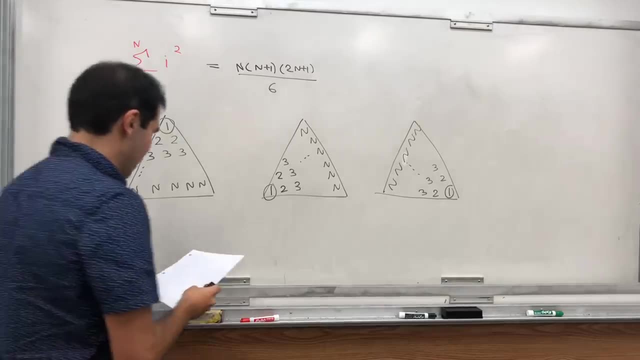 all right, we showed you all right. so the line u came to peak is that one minus four times essentially less than two is en times plus five comes to plus five, not right way. so in total, what we did is we were taking one detail and increasing it, so I gotta make sure we linked it. so make sure you. 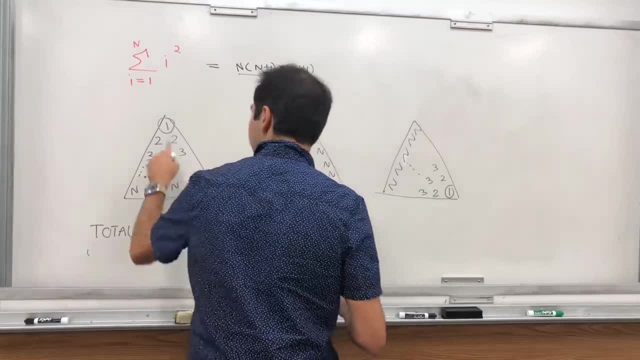 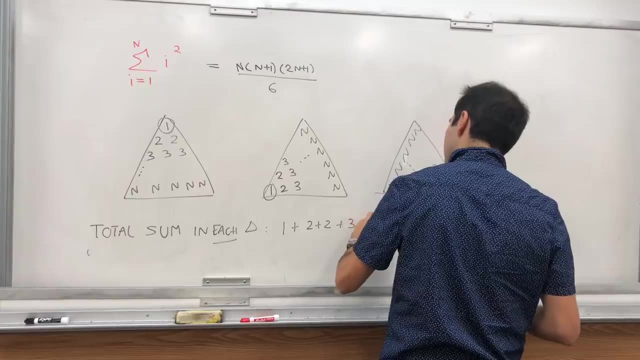 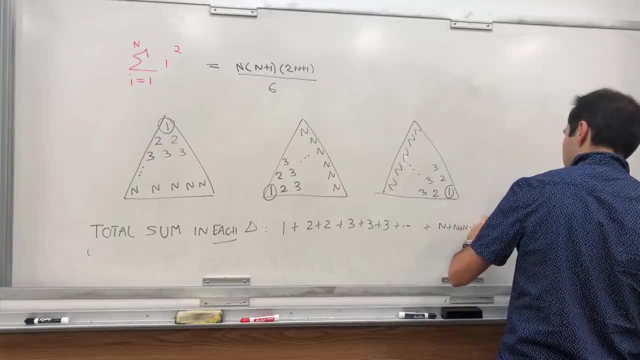 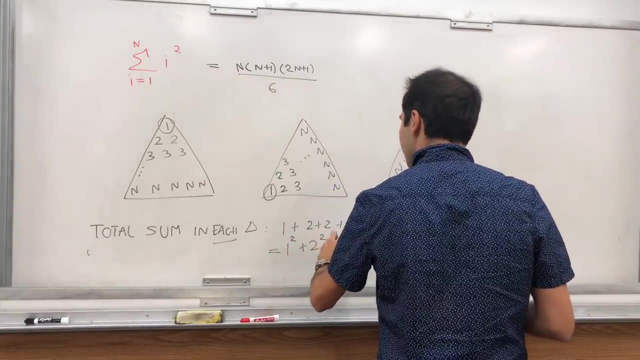 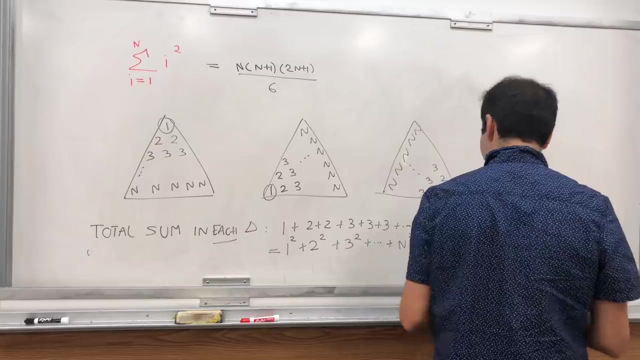 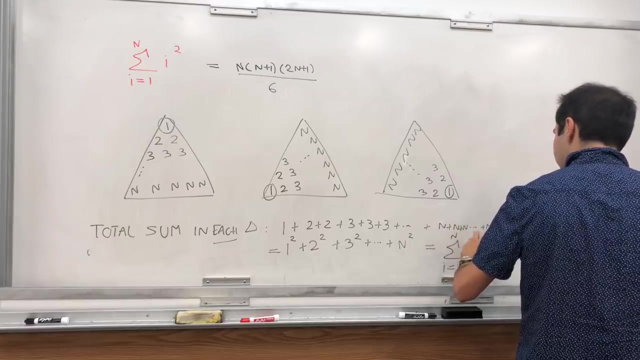 n plus n plus n n times, so which is, if you want one squared plus two times two, which is two squared, plus three times three, which is three squared plus plus n squared, which is precisely what we want: the sum from one to n of i squared and in particular, what this means. 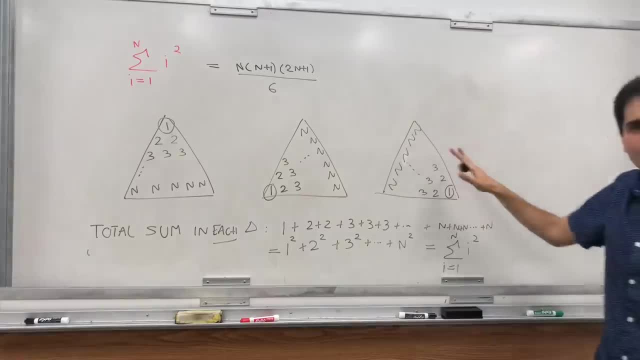 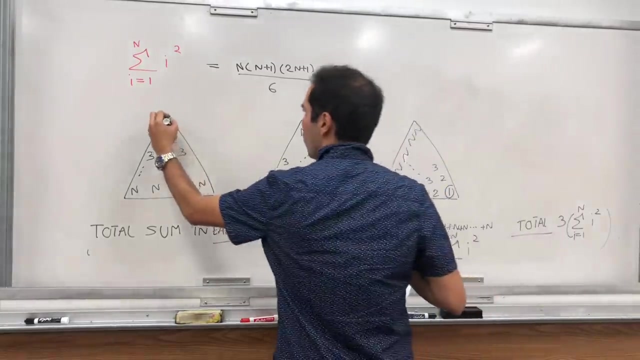 is really the total sum in total is just three times the sum. so the total three times the sum from one to n of i squared. on the other hand, consider summing each term, by which i mean one plus n plus n. that sum would be three times the sum from one to n plus n plus n plus n. that sum would be. 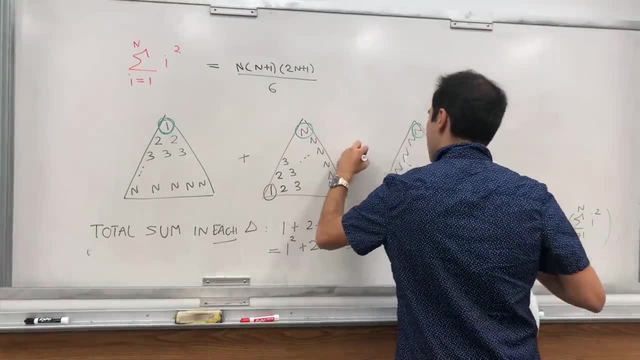 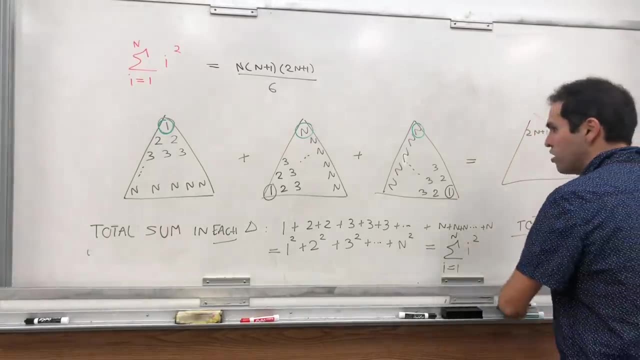 three times the sum from one to n plus n plus n plus n y, three times the sum from one to n plus n plus n, and three times the sum from one to n plus 1,. two times n minus 1 plus one, and let's see what happens here. so 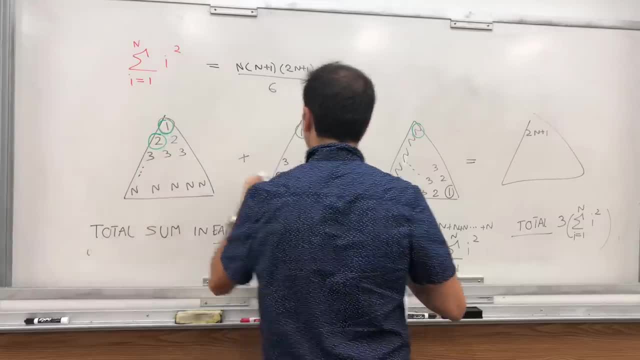 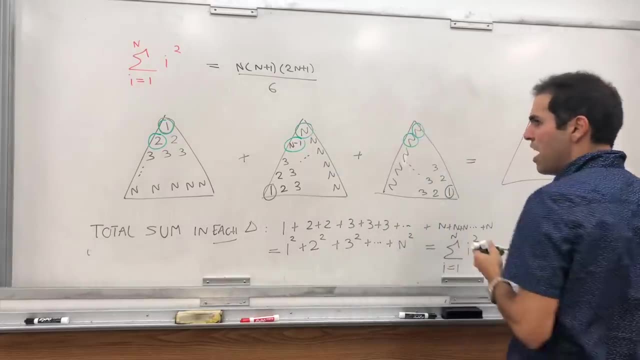 here we have two. let's say two. this term, remember, is like one less. so n minus 1, 2 times n minus 1 plus n. if you sum that up. oh okay, what a surprise. you get 2n plus one, n minus 1 of n squared if you sum that much. 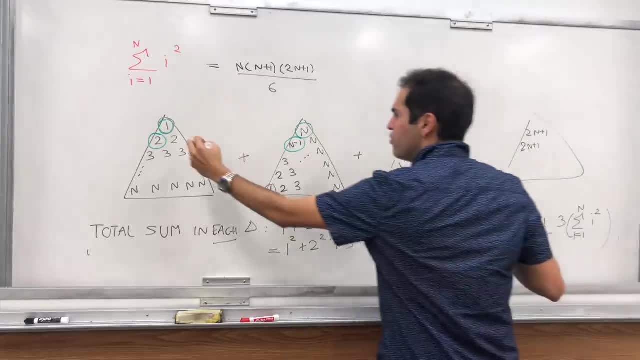 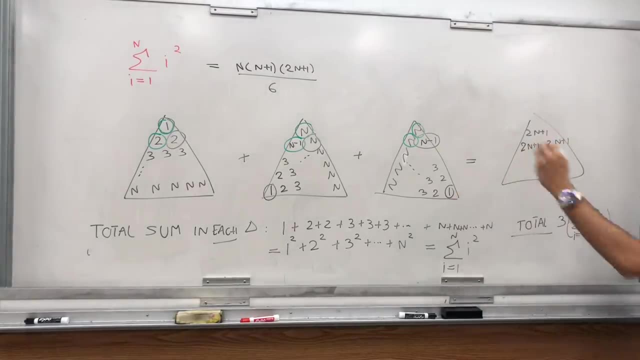 one and same thing. here you have n minus one. if you sum this here, two plus n plus n minus one, you get two n plus one. and in fact it turns out- this is true for every term- two n plus one, two n plus one. and if you don't believe me, let me show you. so what is the i? j term? 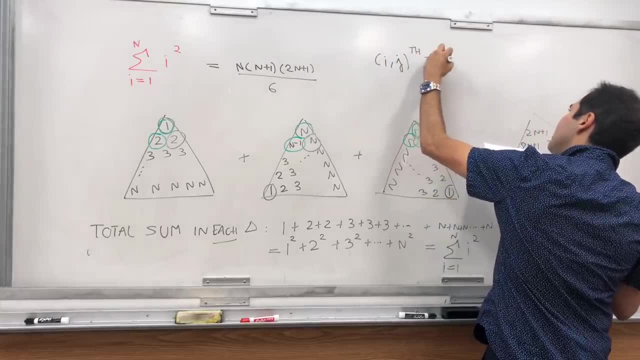 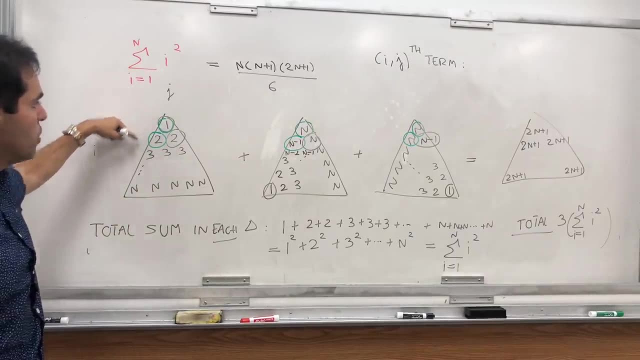 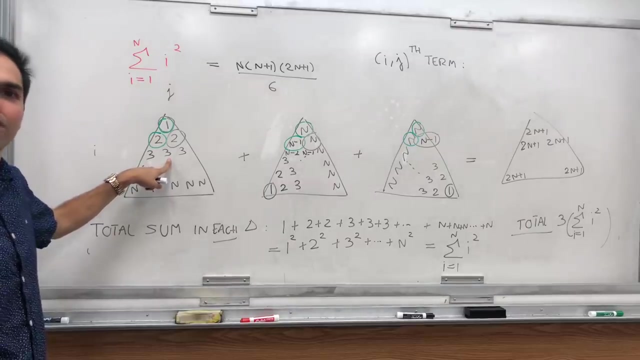 in each thing, so each triangle is different. so, and the i- j term- i mean, for example, the three comma second term- is the term in the third row and the second entry of that, so the j might depend on i, which is okay though. okay, how can we find the entry in the i? jth entry in? 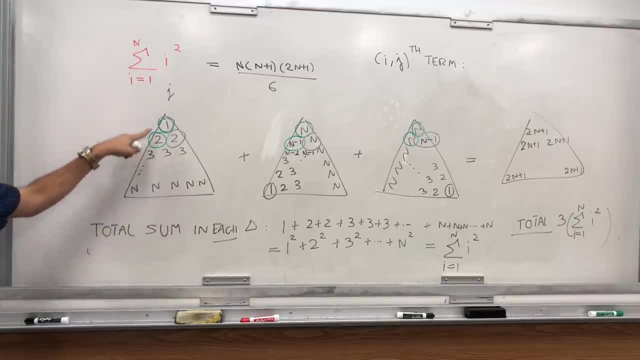 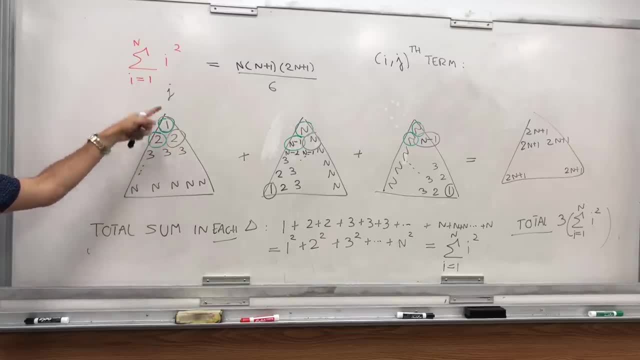 In row 2, all the values are 2.. So the 2 comma j-th entry is still 2.. And also here in row 3, the 3 comma j-th entry is 3.. So in row i the i- j-th entry is i. 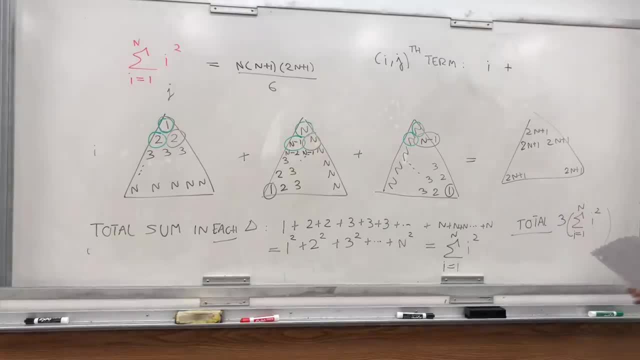 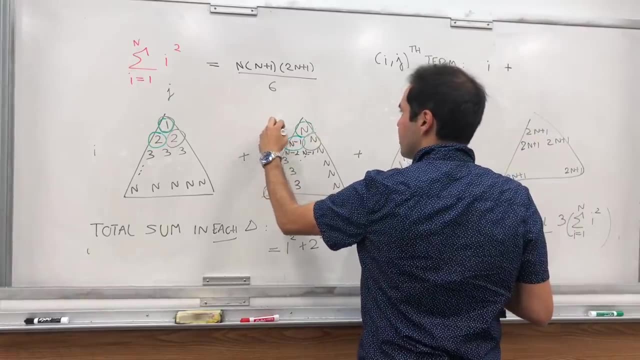 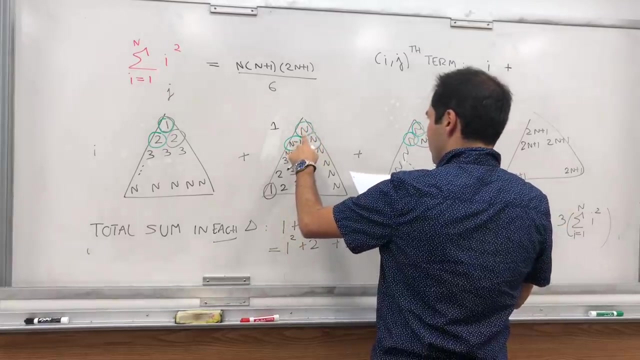 First of all, we have this Now. for this one it's slightly more complicated Because, notice, what we have here is in the first row, let's say row i. the first entry is n, which is really n minus 1. 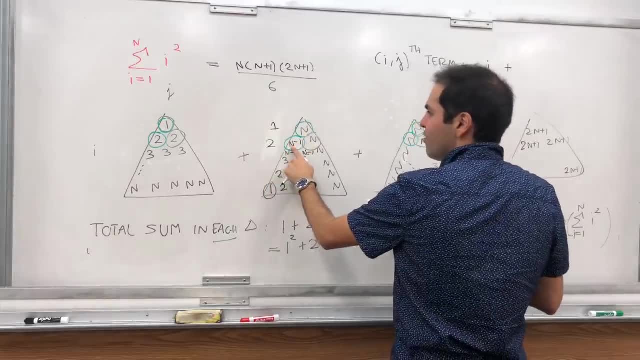 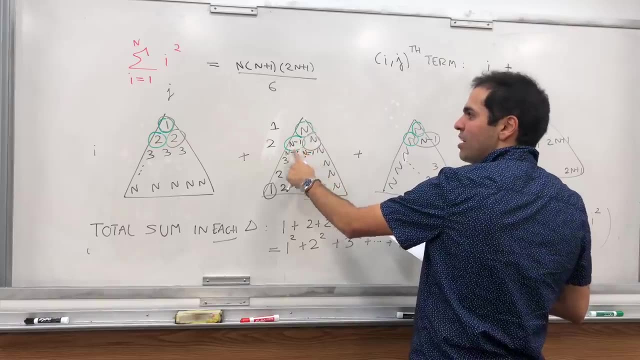 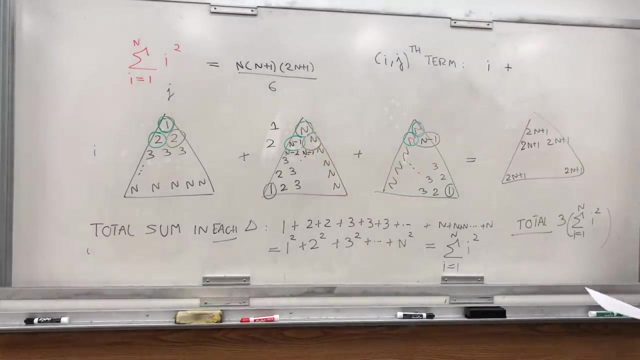 plus 1.. In the second row the first entry is basically n minus 2 plus the 1,, which is n minus 1. But the second entry is n minus 2 plus 2.. So it depends on the row and the column. 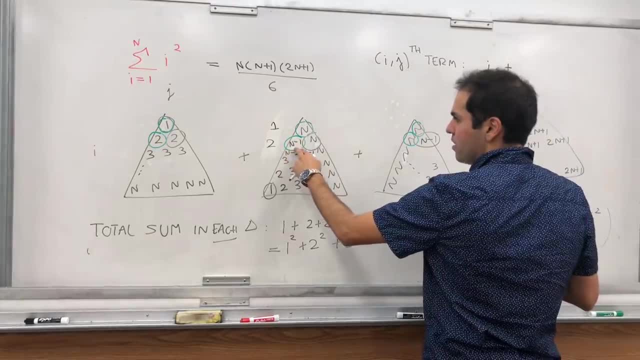 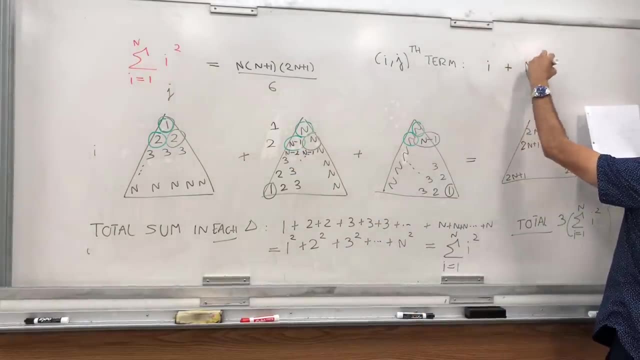 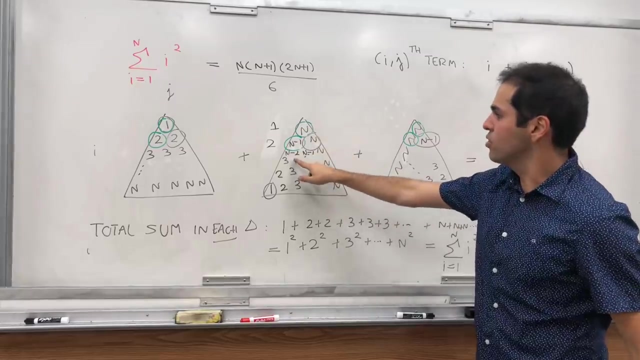 And in general, you see what we have. We have n minus 1, which is 1 less than the row, So n minus i minus 1.. But then you have to add whichever column you're at. So here, for example, in the third row, 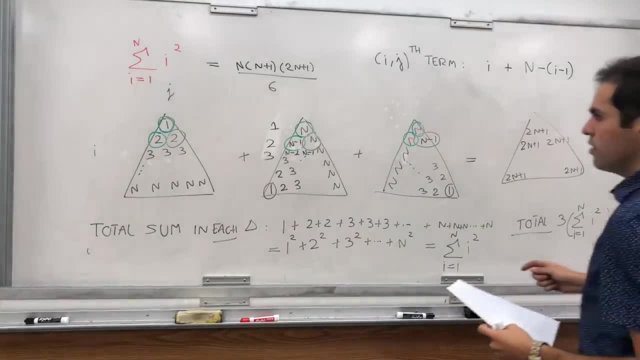 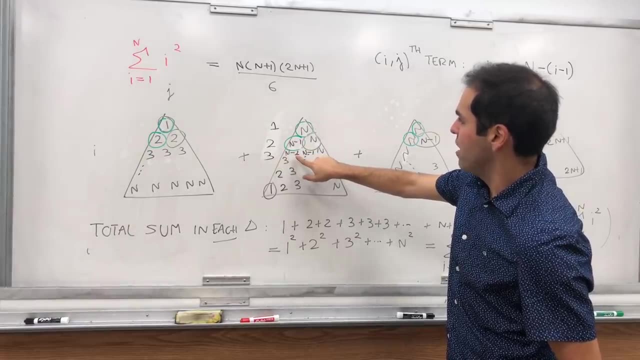 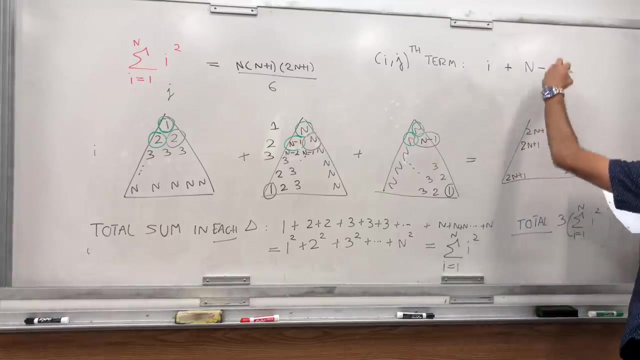 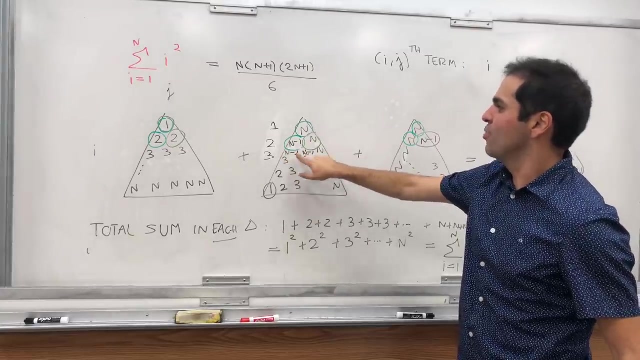 you have to add: We have n minus 3.. And then the first one becomes n minus 2.. So I wanted to say sorry, it's n minus i, So n minus 3, the first one becomes n minus 3 plus 1.. 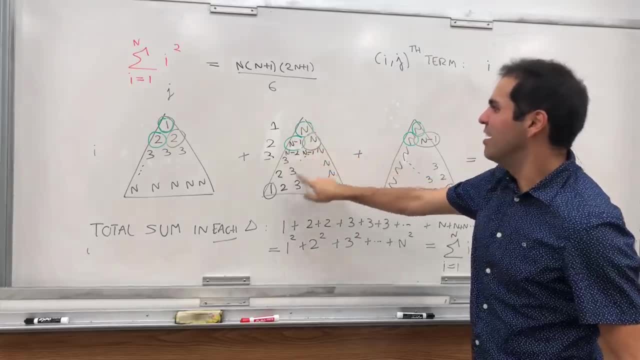 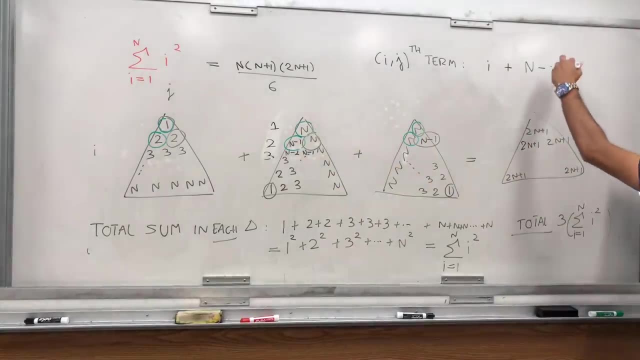 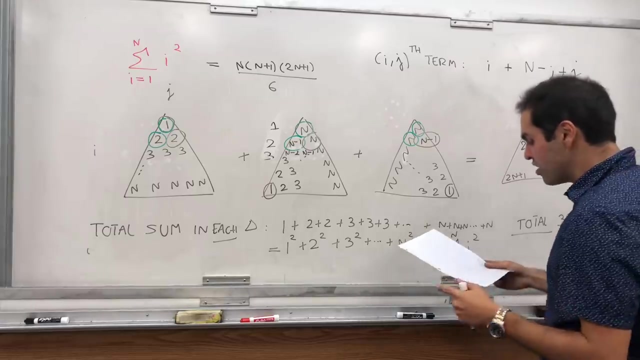 The second term becomes n minus 3 plus 2, up to the third term becomes n minus 3 plus 3.. So in general we have n minus i plus j. This gives us the second triangle. And lastly, for the third triangle, 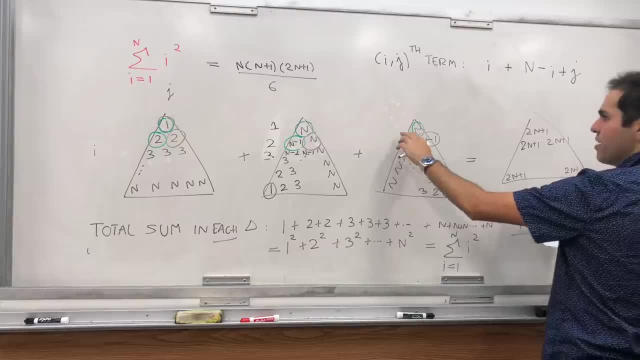 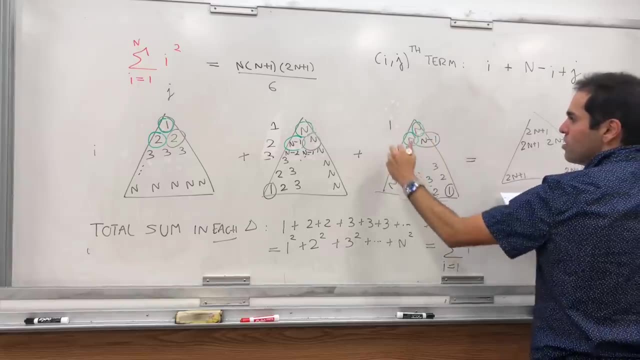 I think it doesn't matter which row we are in, Because look in the first row, well, the first entry is n minus 1 plus 1, which is the first entry. In the second one, again, it doesn't matter which row we're. 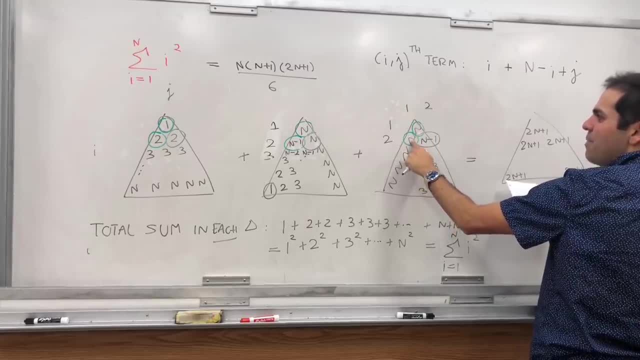 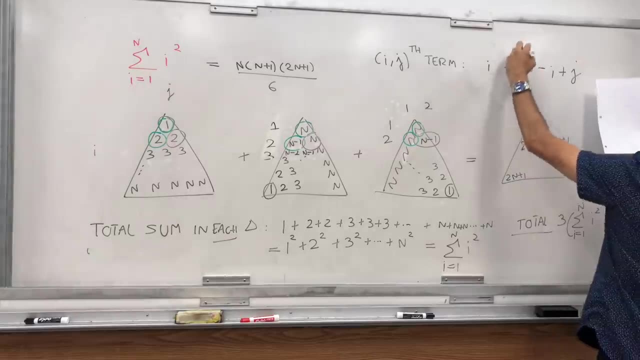 at. It just matters the column. So we have n minus 1 plus 1.. Here n minus 2 plus 1, et cetera, et cetera. So the third one would be n minus j plus 1.. 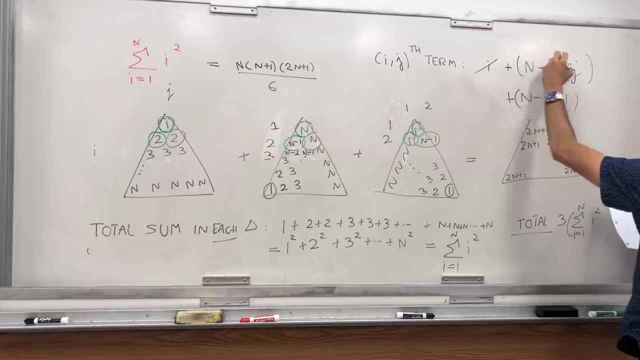 And notice, if you add those up, the i's cancel out, the j's cancel out and you have 2n plus 1.. So, indeed, we have each term. So each term term in each triangle sums up to 2n plus 1.. So how many terms we have? We have well. 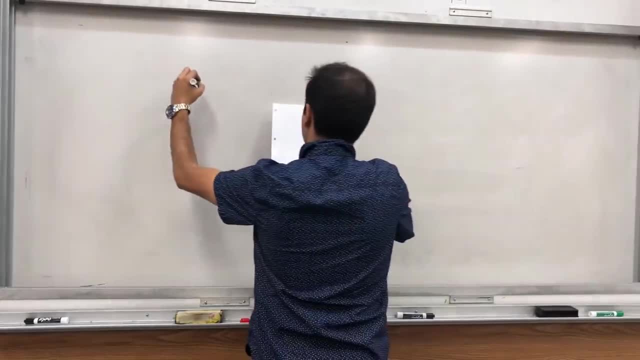 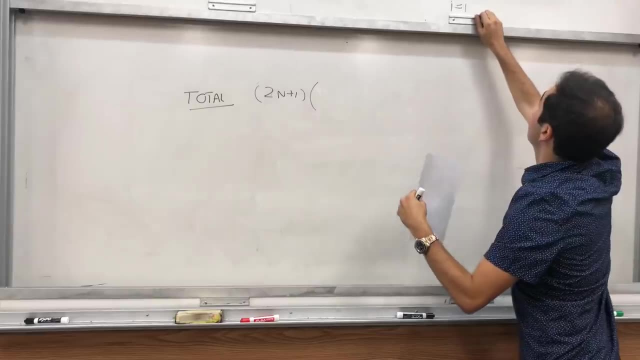 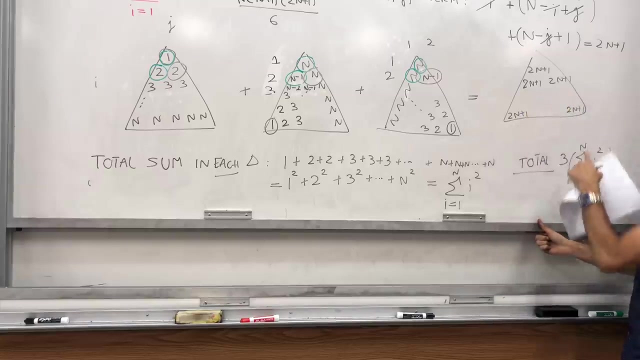 2n plus 1, so total is also 2n plus 1.. And then let's see how many terms are there: 1 plus 2, plus 3 plus 4 up to n. So in other words, the sum from 1 up to n. 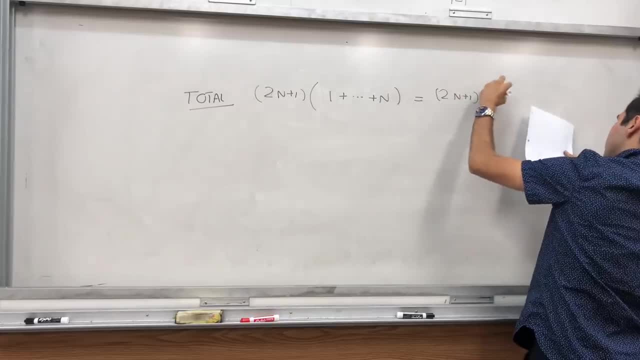 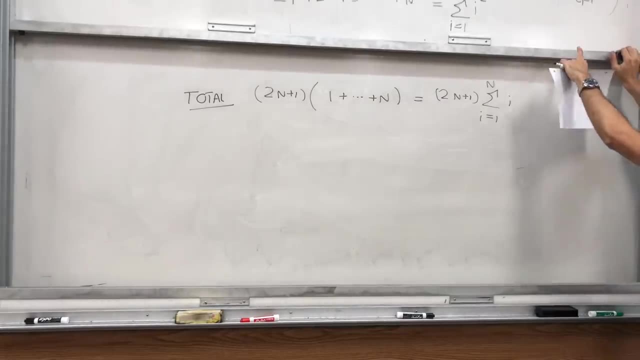 Which is 2n plus 1 times the sum from 1 up to n of i. So what do we have? The total, which is this: 3 times the sum that we want, equals to 2n plus 1 times the sum. 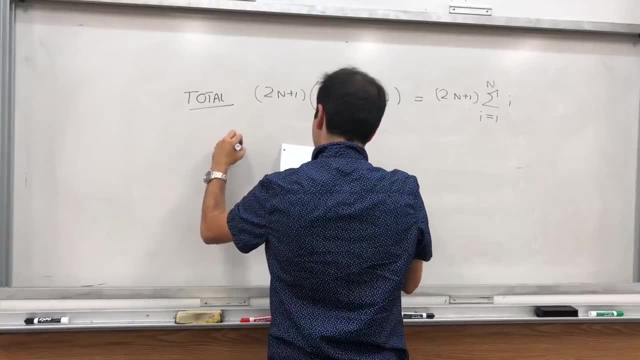 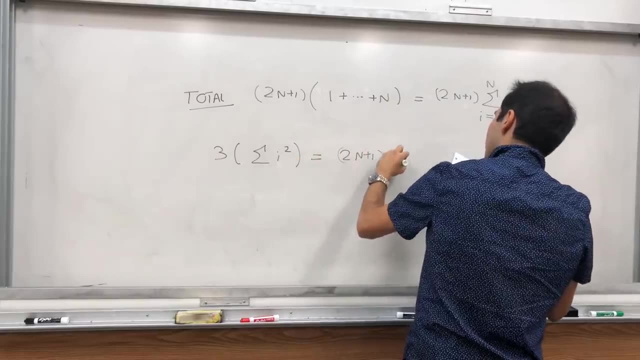 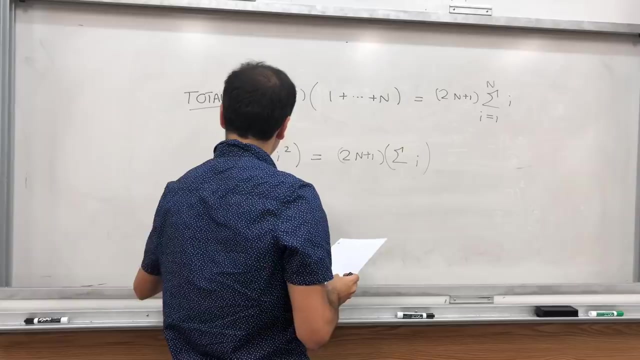 of i's. So indeed, we then get that 3 times the sum of i squares equals 2n plus 1 times the sum of i, And therefore the sum of i squares from 1 to n is 2n plus 1 over 3 times the sum of i. 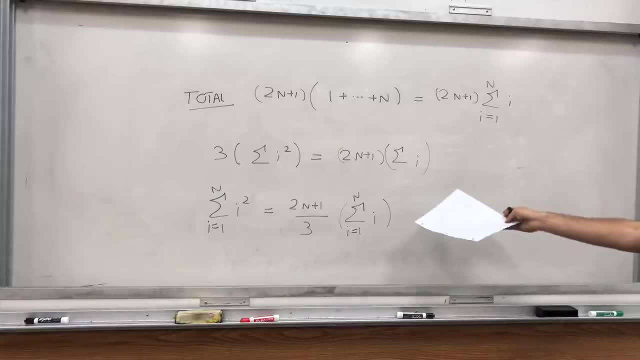 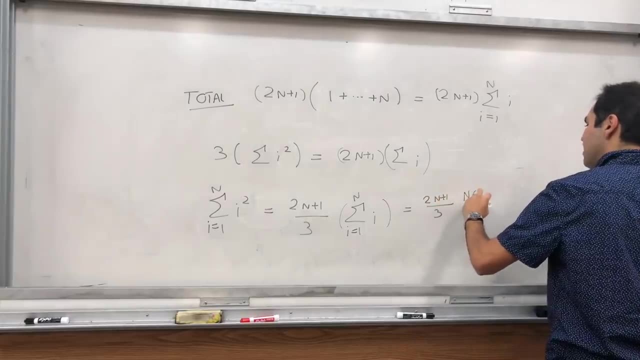 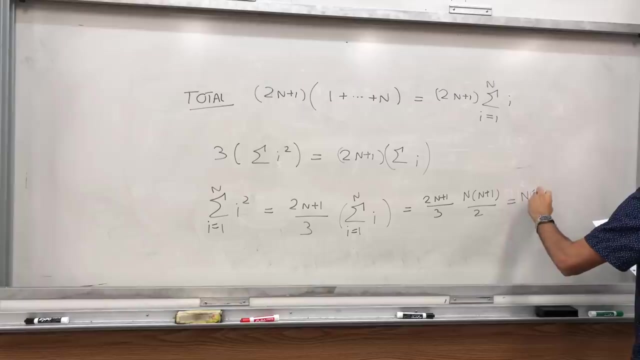 But the sum of the integers- and I want to show it at the end- is simply 2n plus 1 over 3, and then n times n plus 1 over 2.. And if you just multiply all those things, precisely what you want- n times n plus 1 times 2n plus 1,. 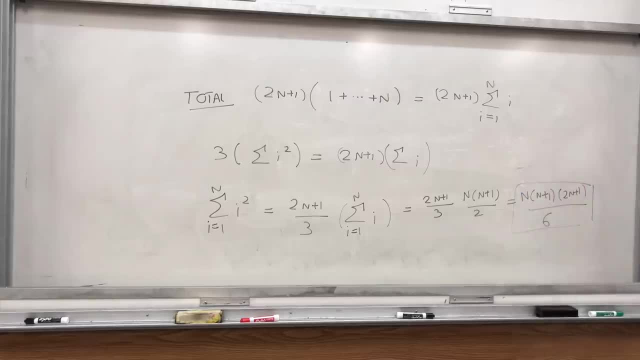 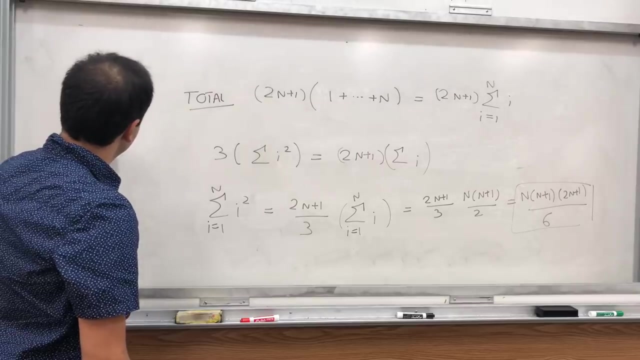 over 6.. How cool is that? No induction required, It just requires counting elements in three triangles. So this is so cool And thank you, Sho. And in case you're wondering where this formula comes from, very quick proof. On the one hand, you consider the sum from 1 plus n.